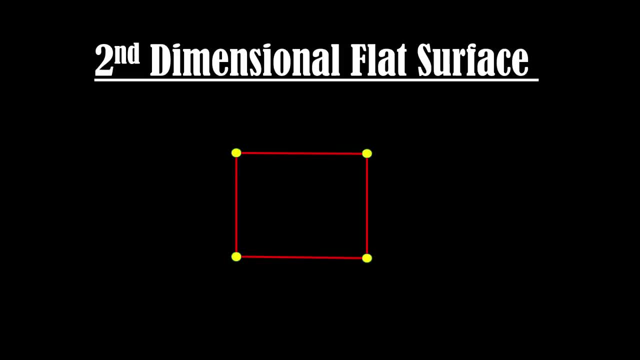 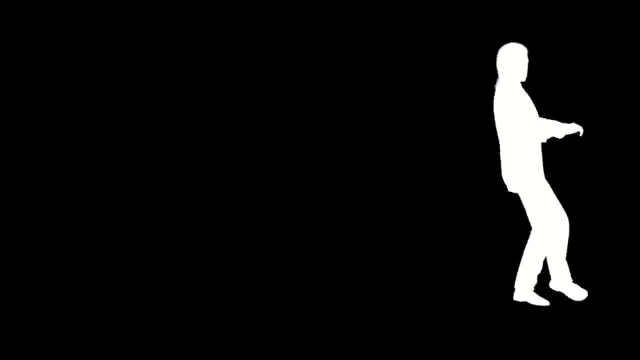 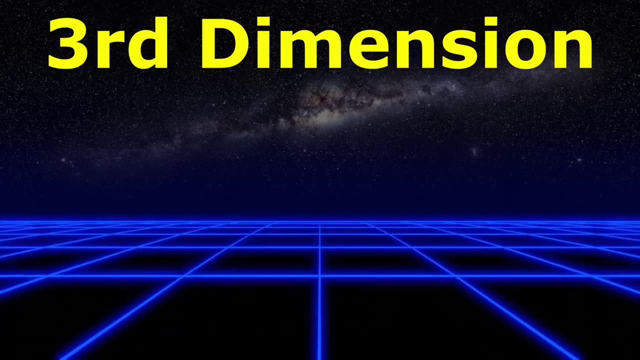 line. Second dimension: Second dimensional or 2D objects are flat shapes like squares and triangles. Motion of a two dimensional being is restricted to a plane surface. therefore it cannot move upward or downward. Third dimension, Third dimensional objects have three dimensions: length, breadth and height. 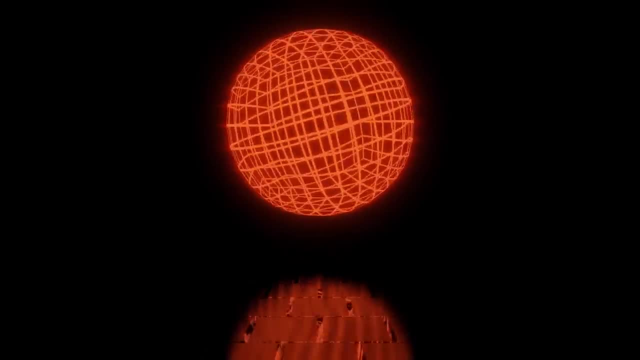 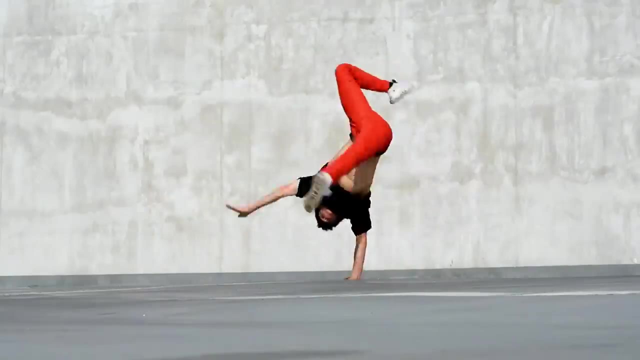 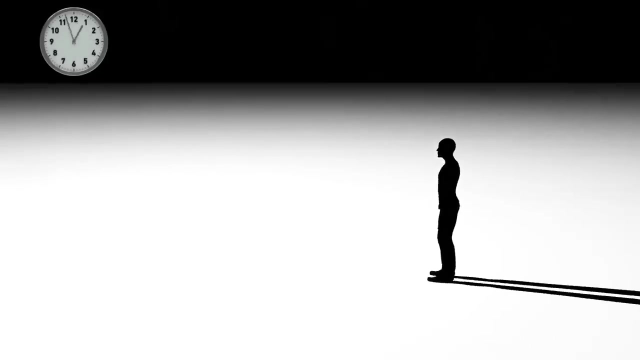 Solid objects like cubes and spheres are examples of 3D objects. We humans are three dimensional beings as we can move freely in three dimensional space. Fourth dimension, Time, is considered the fourth dimension. A four dimensional being can move freely in time dimension and has full control over time. He would be able to move. 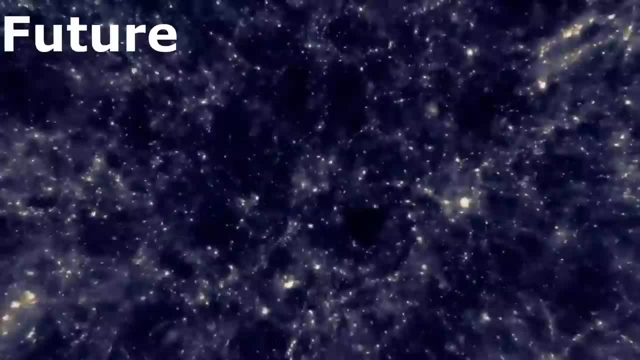 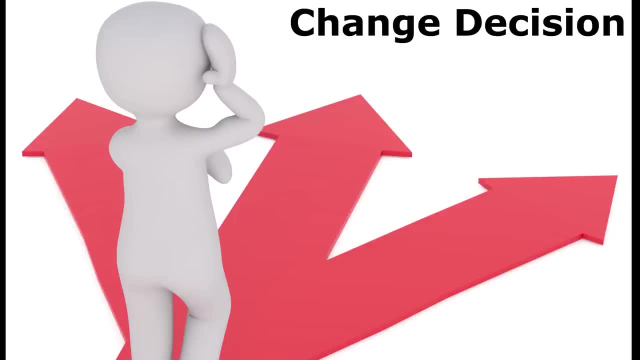 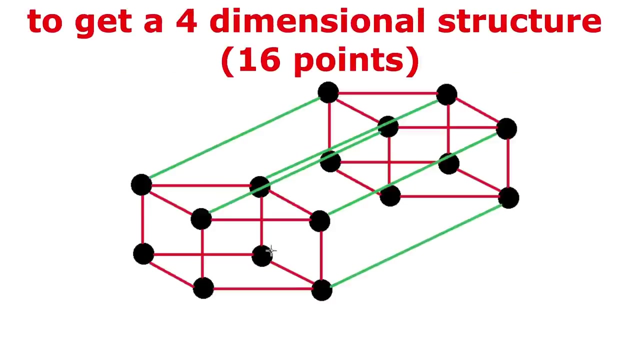 any desired direction in time, past or future. A person living in the fourth dimension can go to a certain point in past time and change its decision. But if we consider the fourth dimension from the geometrical point of view, then hypercube is a four-dimensional object. It is also called 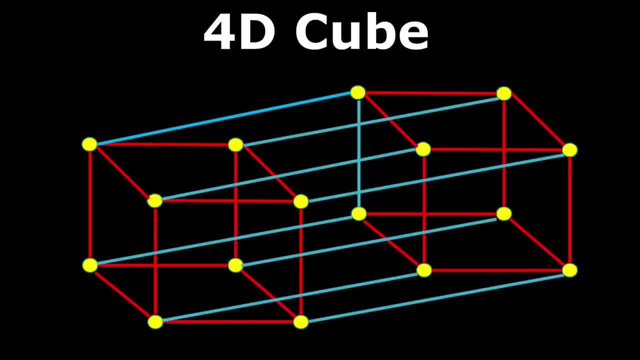 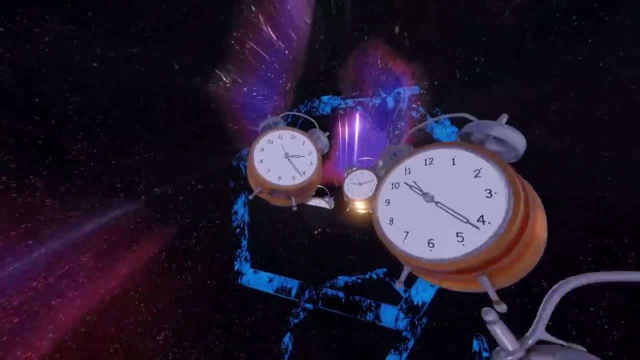 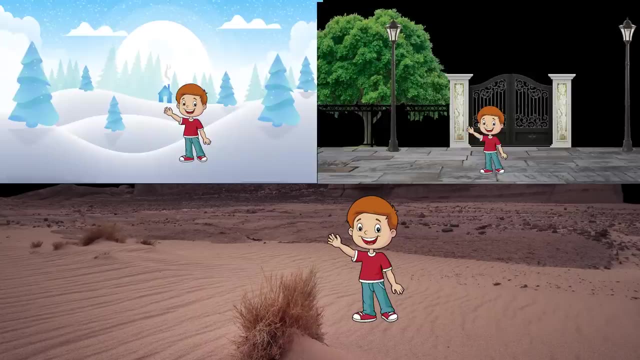 a tesseract. A hypercube is four-dimensional analog of the cube Fifth dimension. A fifth dimensional being can move freely in time, either in past or future, as per his wish, and is able to be present at different locations at the same time. He can do many jobs and have different hobbies. 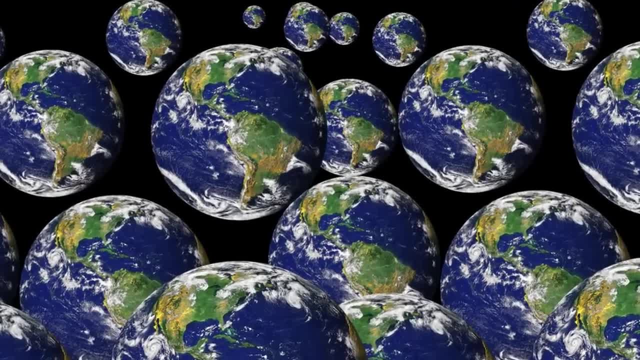 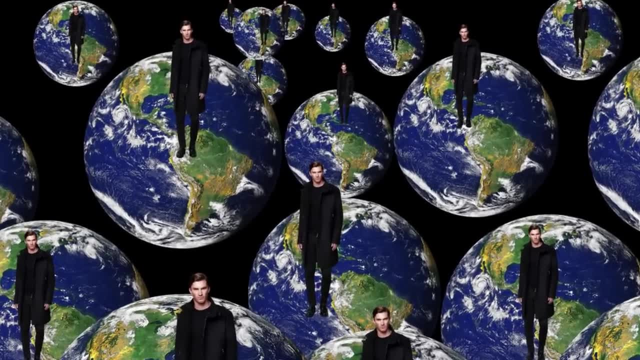 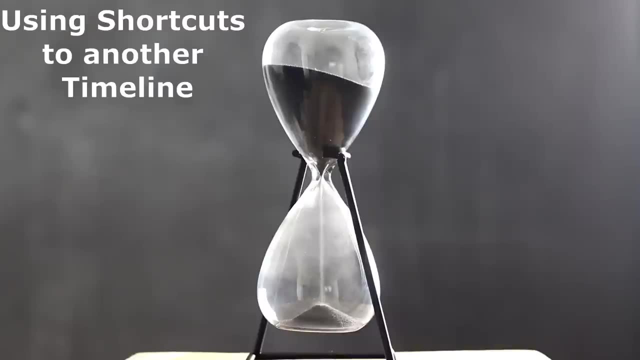 simultaneously. Actually, parallel universes exist in the fifth dimension. Therefore your separate versions can exist in parallel universes having separate timelines. But one limitation of fifth dimension is that you cannot meet your self version Directly by using shortcuts to another timeline of parallel universe. Sixth dimension: In the sixth, 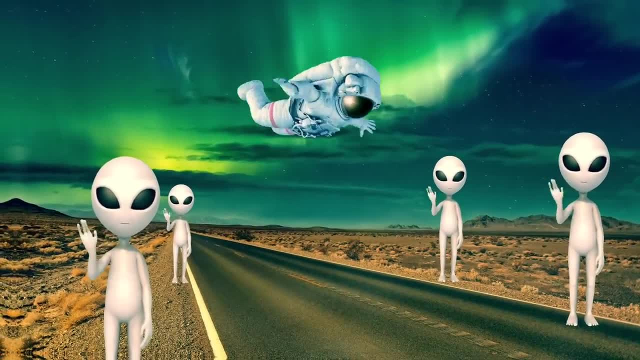 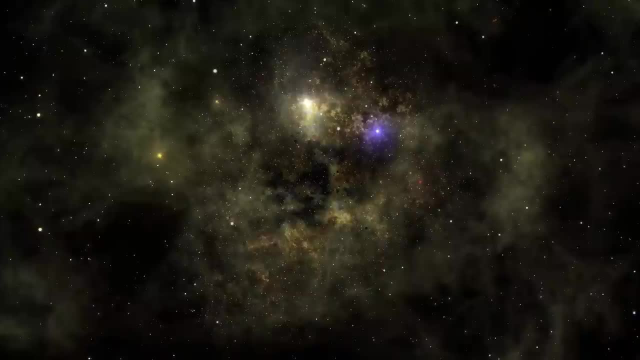 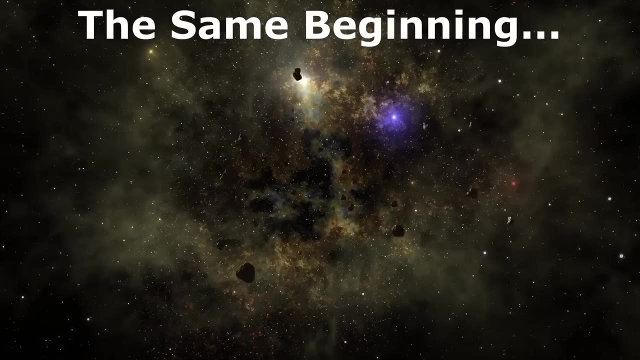 dimension you have all the powers that you possess. in the fifth dimension You can see all the presents, pasts and futures of all the parallel universes. But one limitation of the sixth dimension is that all the parallel universes must have the same beginning or the initial condition. 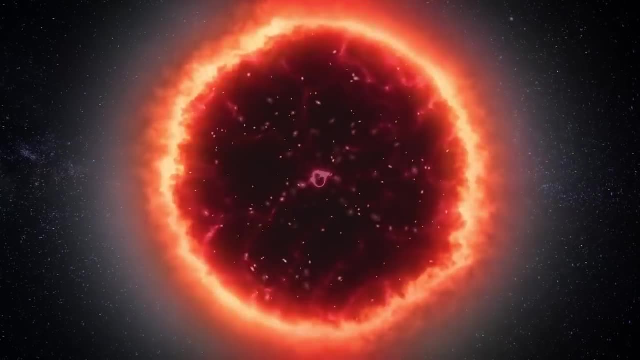 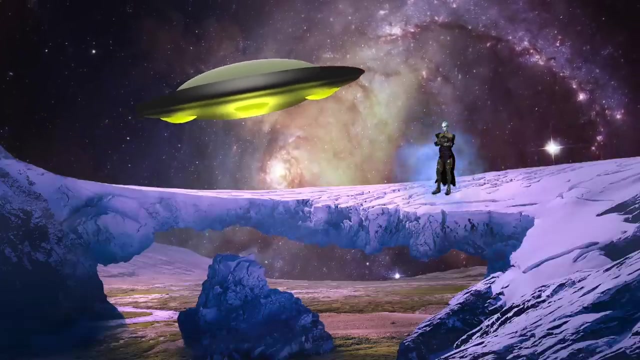 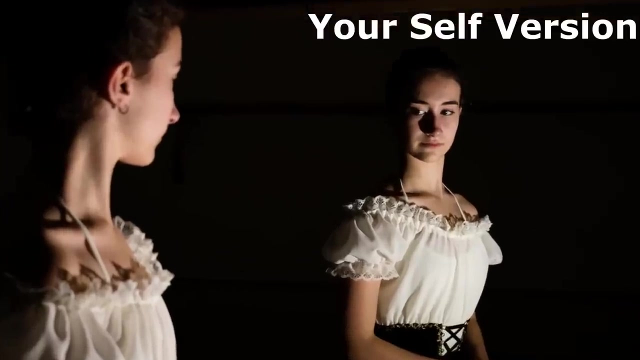 that is the Big Bang. But in the sixth dimension you are free from the limitations of the fifth dimension, as you can easily jump from the timeline of your universe to any point present on the timeline of any parallel universe and meet your self version. In the sixth dimension, your multiple versions can live their lives in parallel. 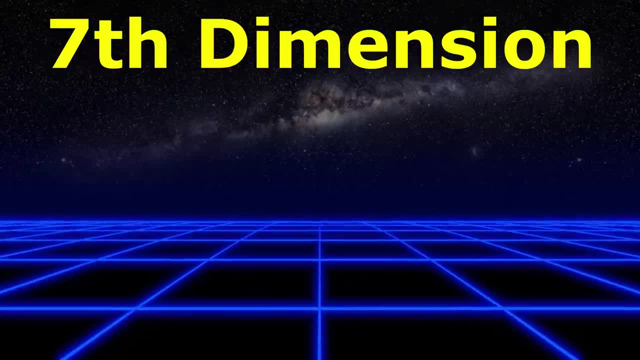 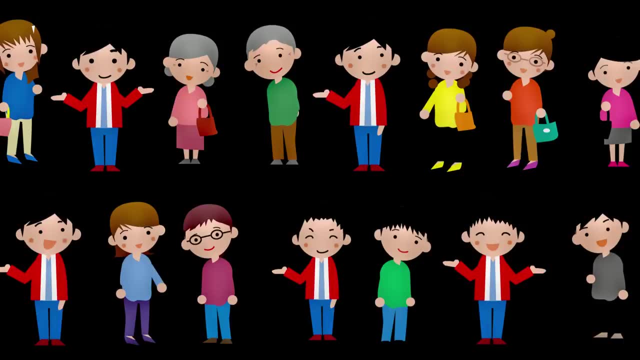 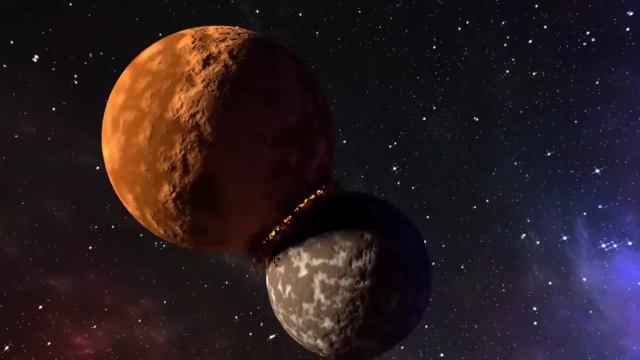 universes simultaneously. Seventh dimension. All the powers of a sixth dimensional being are possessed by the being of seventh dimension. He can have forms of itself and can move from one universe to any other universe. Unlike the 6th dimension, the 7th dimensional universes may have originated from different start conditions. 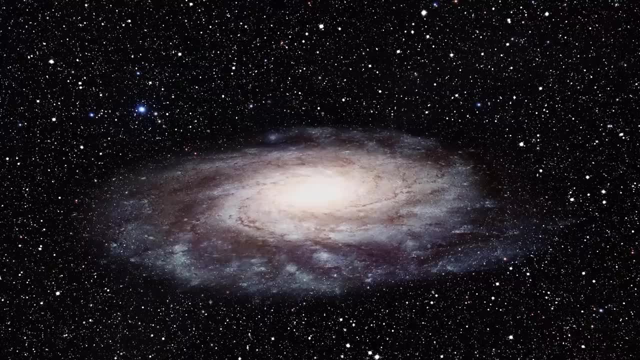 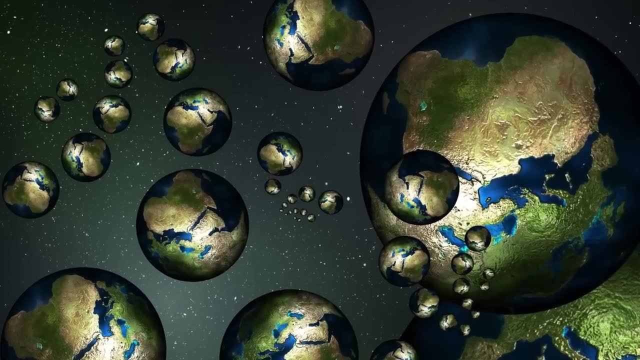 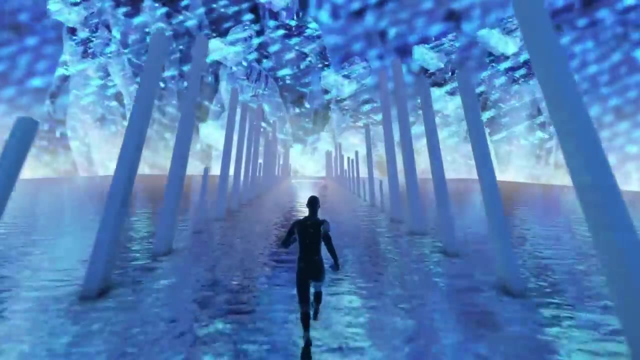 not just the Big Bang. 8th dimension. The 8th dimension has a plane of all the possible presents, pasts and futures, for all the infinite number of parallel universes. According to the theory, in the 8th dimension objects do not have any physical existence, like our digital world. 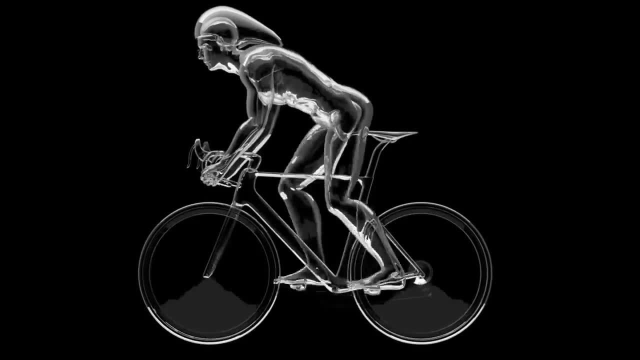 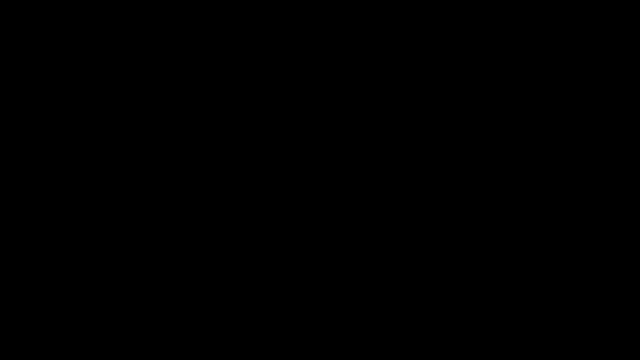 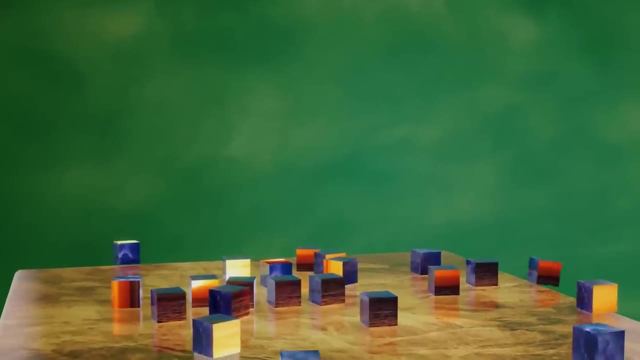 where we cannot touch the objects but only can see or hear them. In the 8th dimensional world, things can change shapes, size and appear or disappear instantly, somewhat like the virtual reality. 9th dimension: In the 9th dimension, universes may have their own laws of physics. 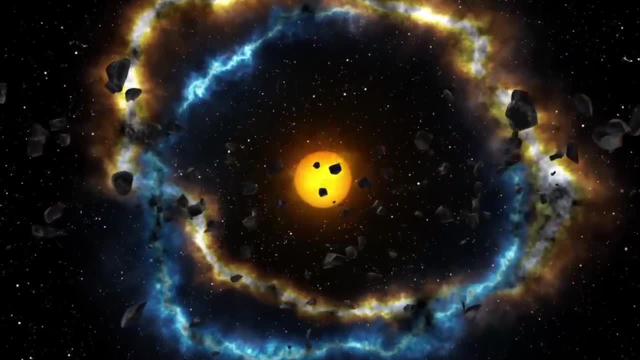 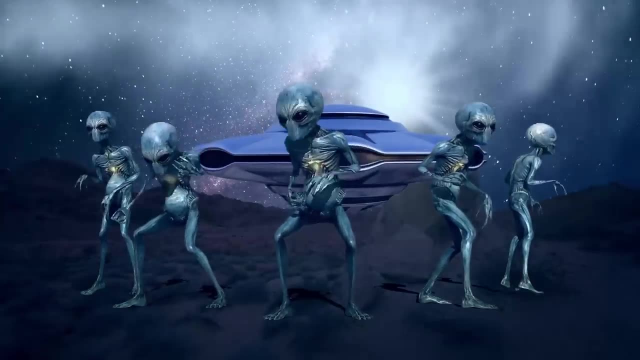 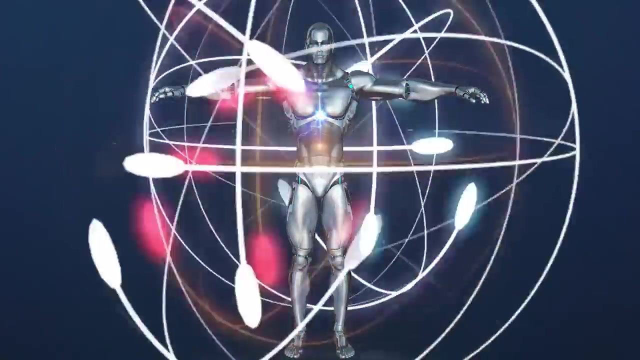 and separate conditions and problems of their origin. Surprisingly, in the 9th dimension, many civilizations or aliens may live simultaneously at the same place. These coexisting civilizations may not see or feel the presence of each other. The superpowers of a 9th dimensional being will blow your mind. 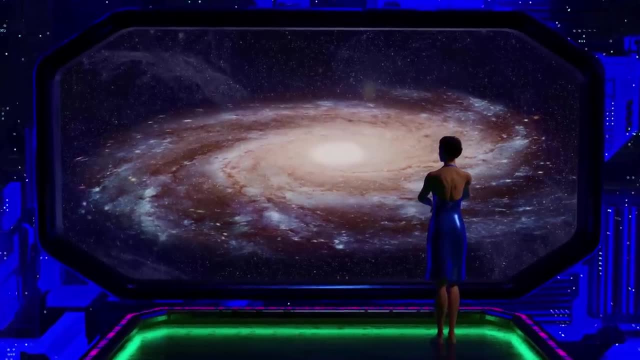 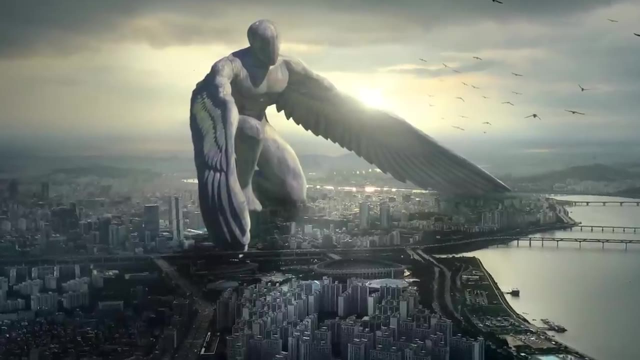 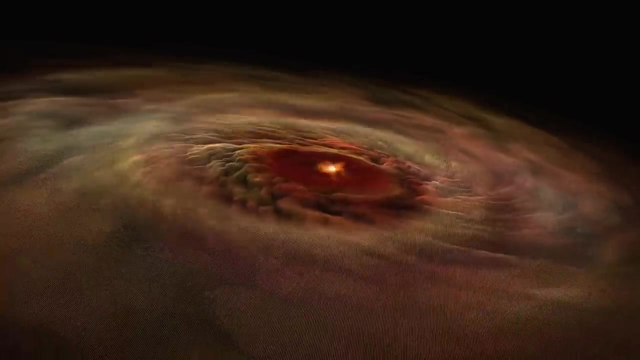 He would have no physical form and would be able to move freely in space and time in any of the universes. 10th dimension, His 10th dimensional being, would possess infinite powers that are beyond your imagination. It would be possible for him to control even the space-time and everything present in all the infinite number. 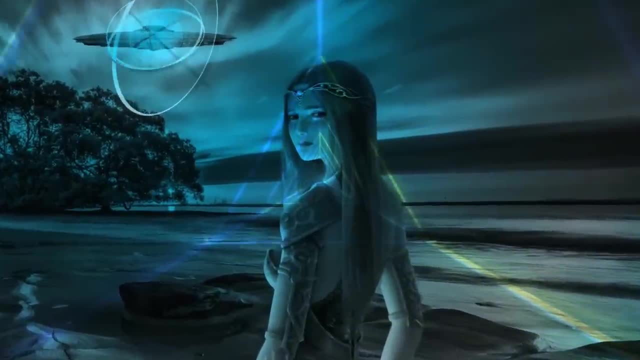 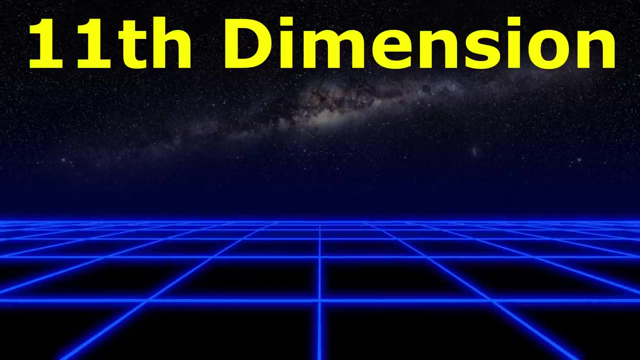 of universes Because of the infinite powers of the 10th dimensional being. some researchers also suggest that the God lives in the 10th dimension. 11th dimension: According to the string theory, everything in the universe is made up of. 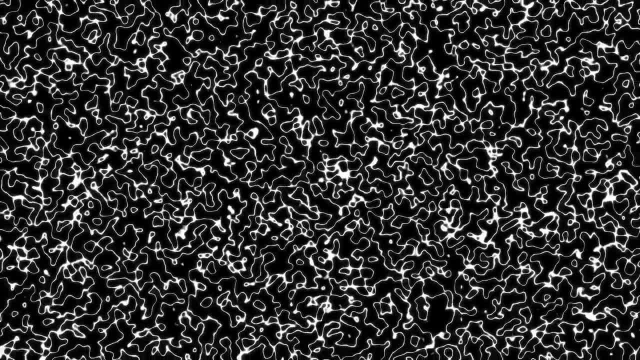 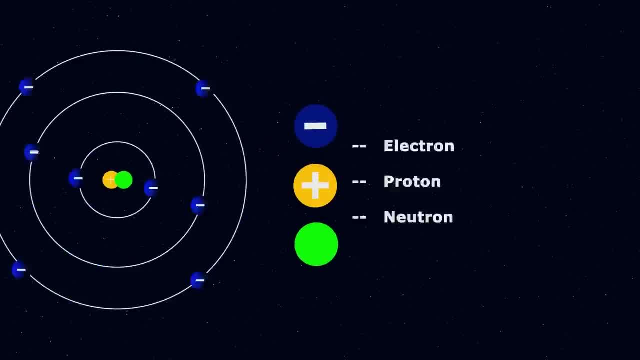 infinity. So How can you predict how light and chaos would be in the space and time of universes? infinitely small, one-dimensional vibrating loops called strings. These strings vibrate in 11 dimensions. Even the subatomic particles like electrons, protons and neutrons are made up.